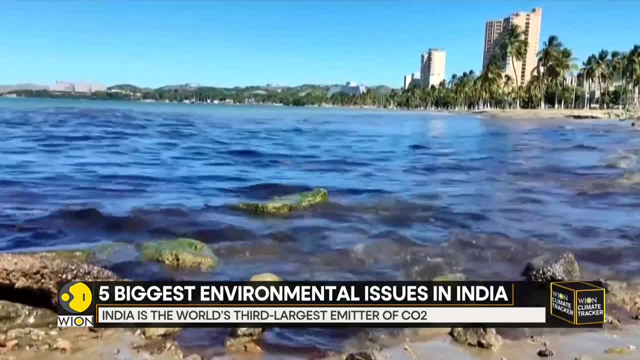 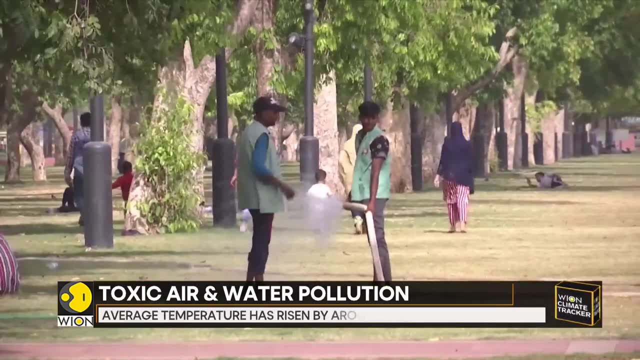 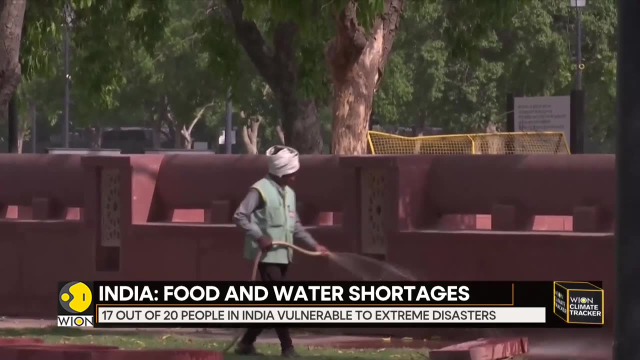 of up to half of GDP growth. Now third on the list is food and water shortages. According to the Intergovernmental Panel on Climate Change, India is the country expected to pay the highest price for the impact of the climate crisis. Earthorg, an environmental data. 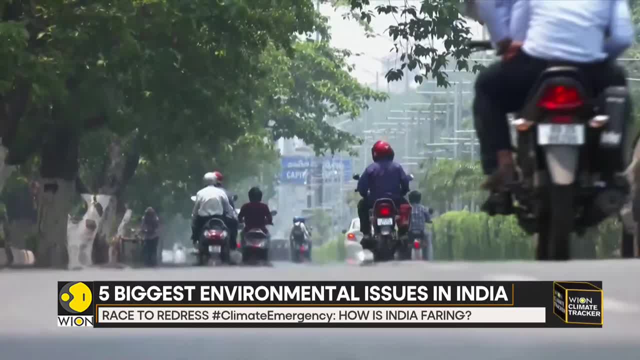 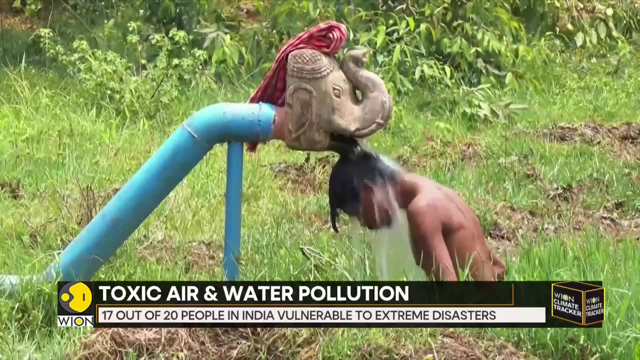 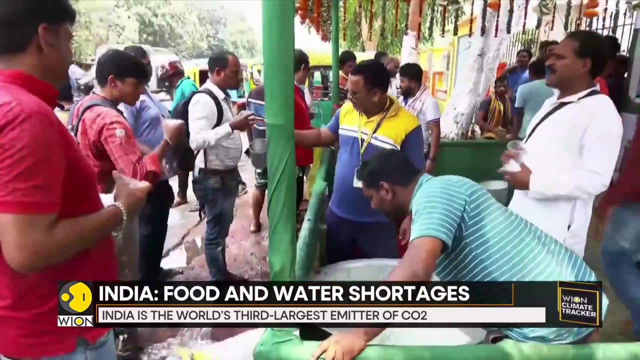 platform says that there is no doubt among experts that unprecedented heatwaves are a direct manifestation of climate change. March 2022 marked the hottest and the driest month recorded in 120 years. India's northwest regions have been dealing with a prolonged wave of scorching. 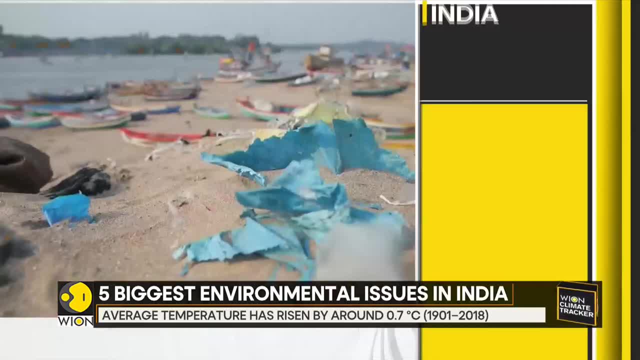 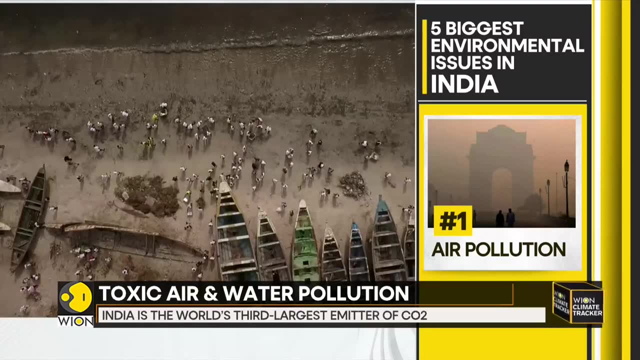 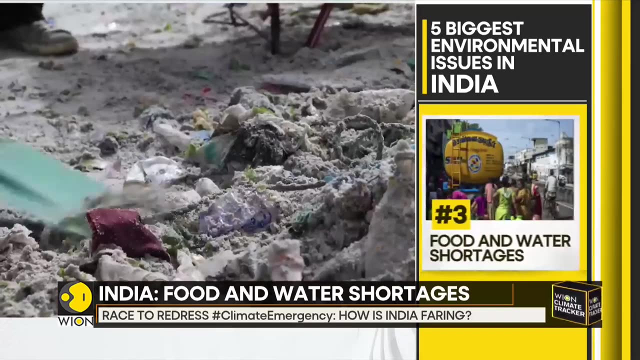 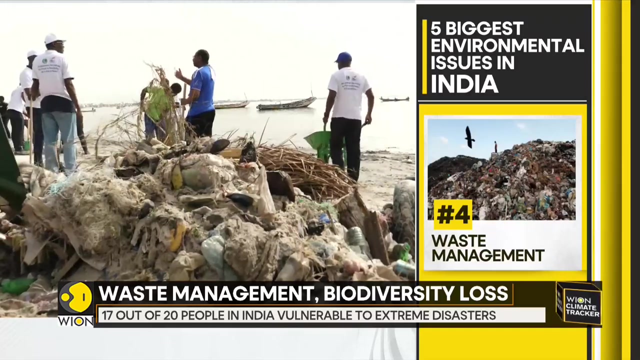 and record-breaking heat. Now next on the list is waste management. As per reports, experts estimate that by 2030, municipal solid waste is likely to reach 387.8 million tonnes and will more than double the current value by 2050.. India's rapid urbanisation makes waste management extremely. 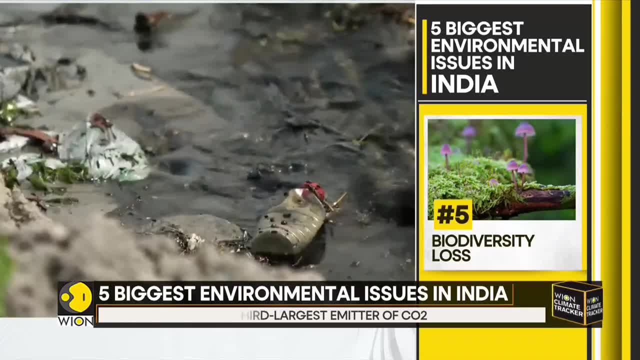 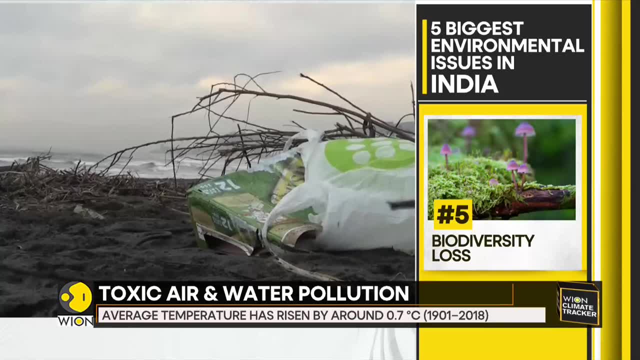 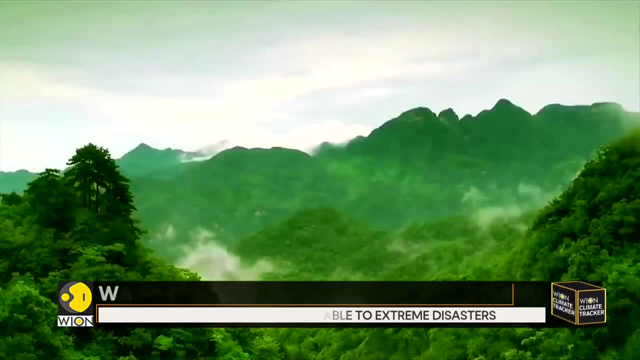 challenging. Currently, about 5% of the total collected waste is reportedly recycled, 18% is composted and the remaining is dumped at landfill sites. Last but not the least, biodiversity loss. India has four major biodiversity hotspots. 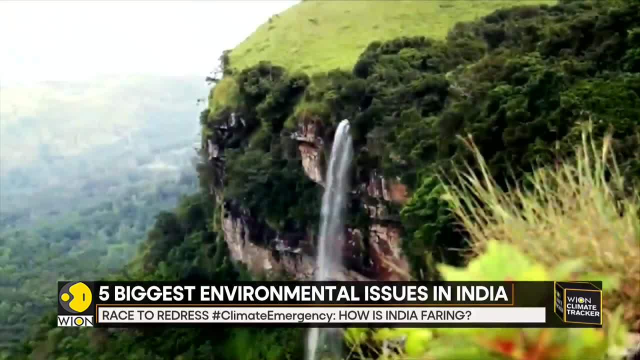 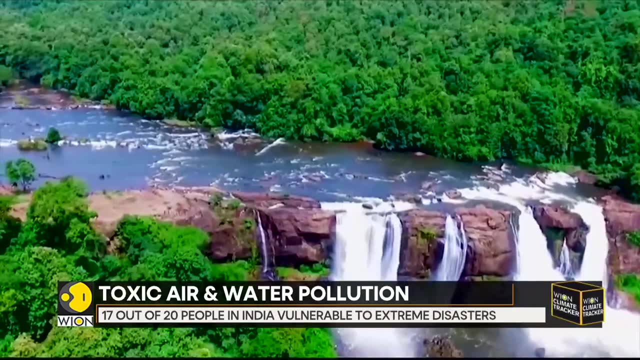 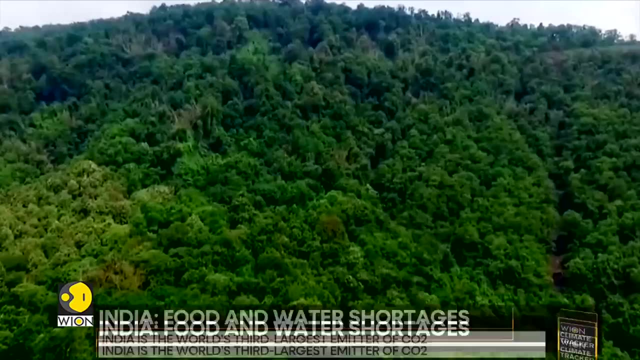 Himalayan desert, India's largest biodiversity hotspot. India's largest biodiversity hotspot players, Western Ghats, Sunderland and Indo-Burma region. These are regions with significant levels of animal and plant species that are threatened by human habitation. More than a thousand animal species in India are currently monitored by the International. 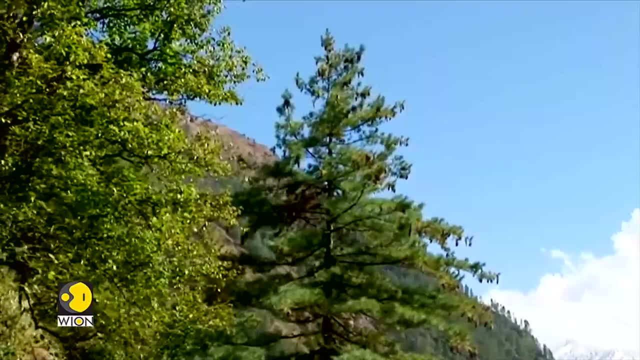 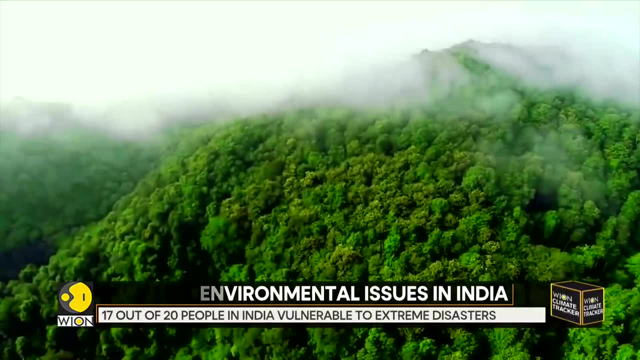 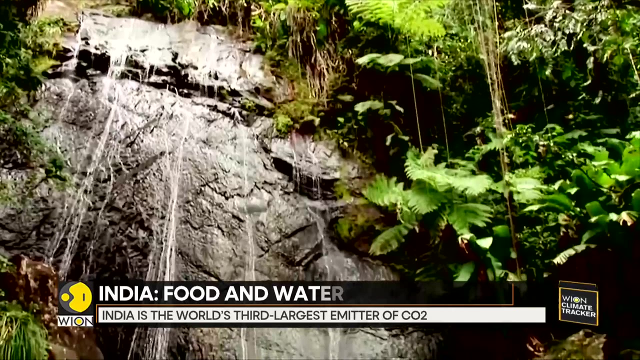 Union for Conservation of Nature Red List. As per WWF and the Zoological Society of London, freshwater biodiversity in India has experienced an 84% decline Since the start of this century. India has lost 19% of its total tree cover. For more UN videos, visit wwwunorg.